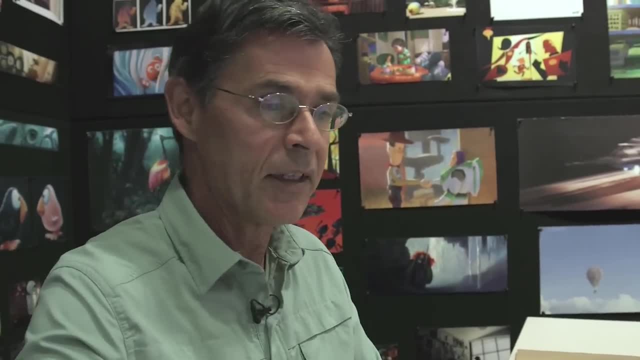 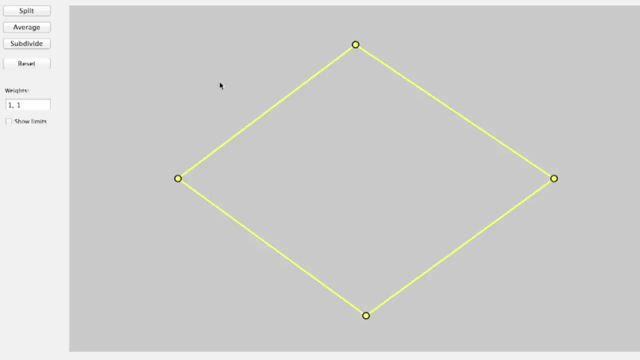 let's start, say, with curves in two dimensions to explain the basics of the process. So what I've got here is a little four point polygon and it's going to be my job to make a smooth curve out of it. I'm going to make a smooth curve out of it by just repeating a few simple steps. So the first: 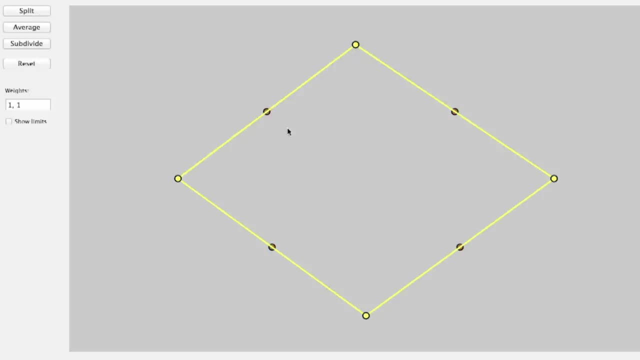 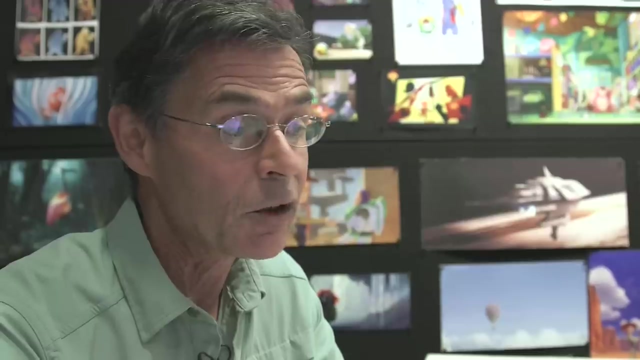 step I'm going to call split, And what that does is it adds midpoints to the edges. So now I've got eight points, but it's not really any smoother. The next thing I'm going to do is I'm going to make it a little bit smoother by repositioning all eight of these points. So this guy, for instance, 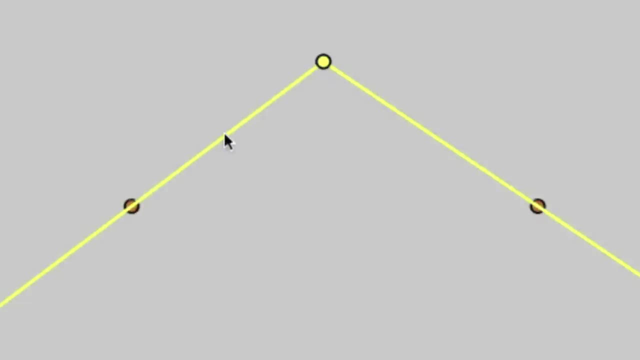 is going to move from where he is now to the midpoint of his right neighbor. This guy is going to move to his right neighbor And let me animate that for you. I'll call that the averaging step. So now I've got eight points a little bit smoother. 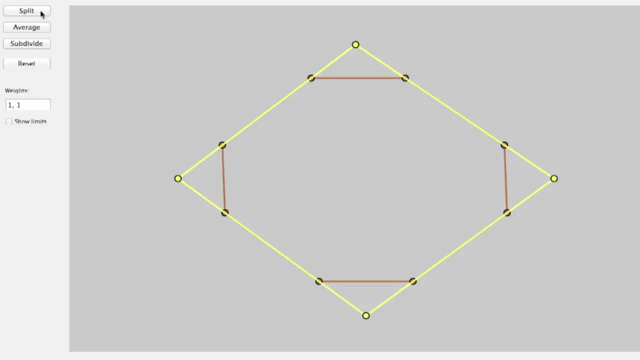 And again, my goal is to make a smooth curve, And so I'm just going to repeat, I'm going to split and average. So now I've got 16 points- Again a little bit smoother. I'll put those two steps into a combined step. I'll call subdivide, And you see that as I 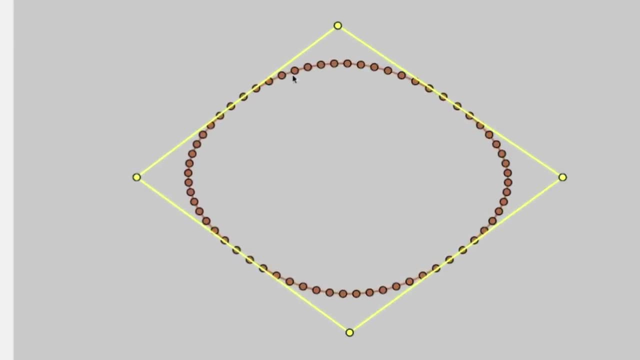 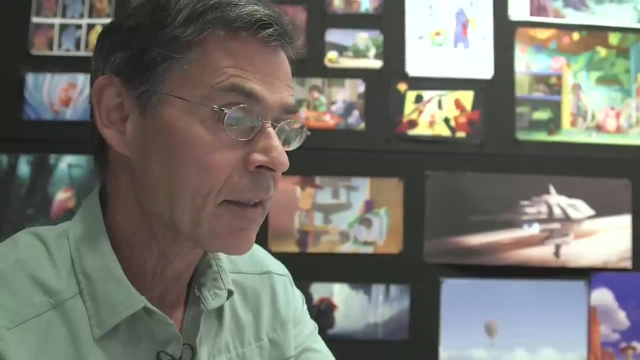 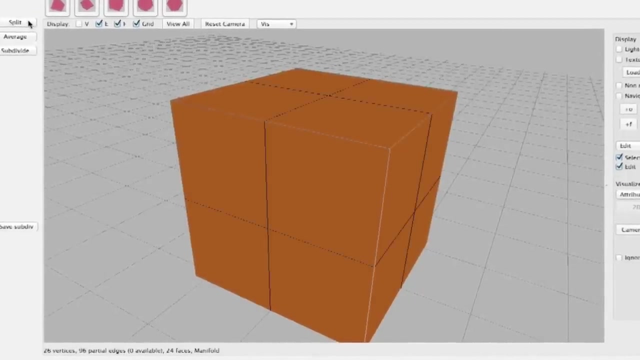 continue to subdivide, the smooth curve starts to emerge, And that's the basis of how we create all of our surfaces. This splitting and averaging idea also works for surfaces. So here's an example where I start with a cube. So if I split, it's a little more complicated for surfaces. 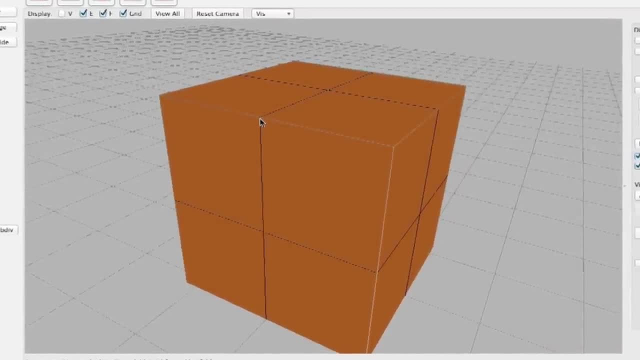 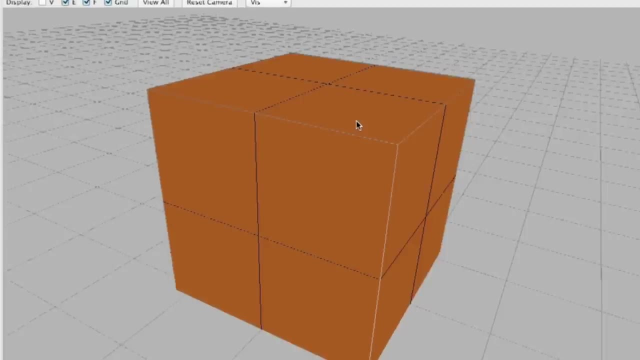 to split, I have to insert edge midpoints like this one here, like I did for curves, And I also have to introduce the middles of faces. But again, that's just done by averaging. So this point here is just the average of the four points around it, And then I average. In this case I need to use a 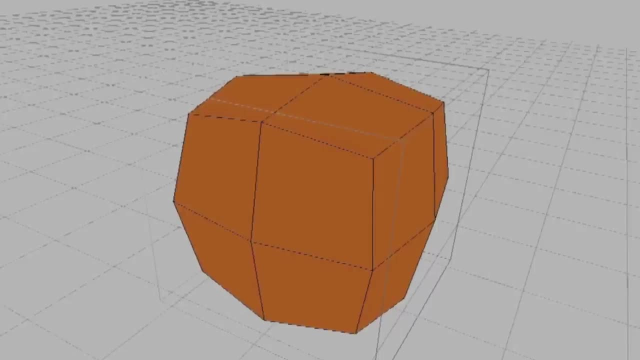 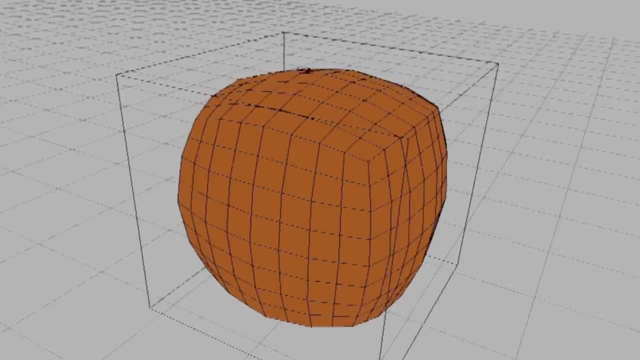 carefully constructed weighted average for reasons we may talk about in a minute. But if I pick my averaging weights carefully enough, I can continue the split and average process and generate smooth surfaces in the limit. And that's exactly how Jerry's hand, and in fact Jerry himself, was built. 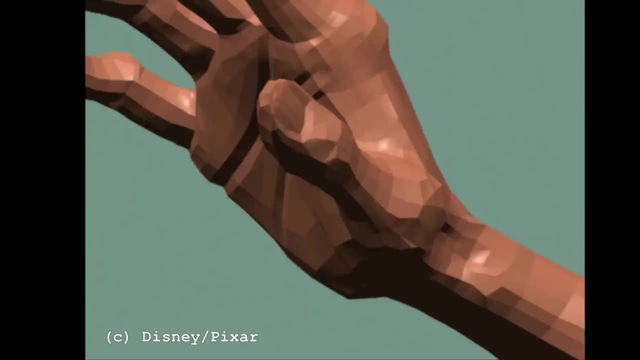 Well, here, for instance, are the points that we digitized off this sculpture Before subdivision. we run this splitting and averaging process a lot of times, And that smooths the surface out and creates the smooth shape that you ultimately see on the screen. 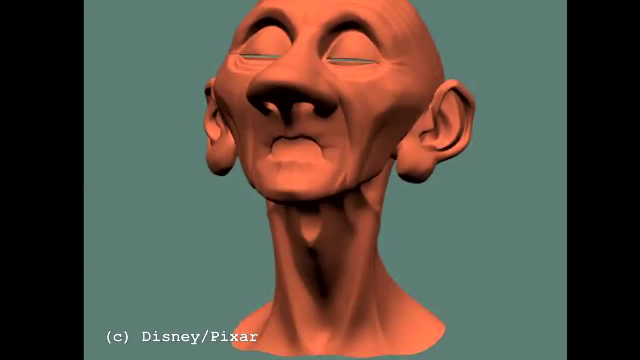 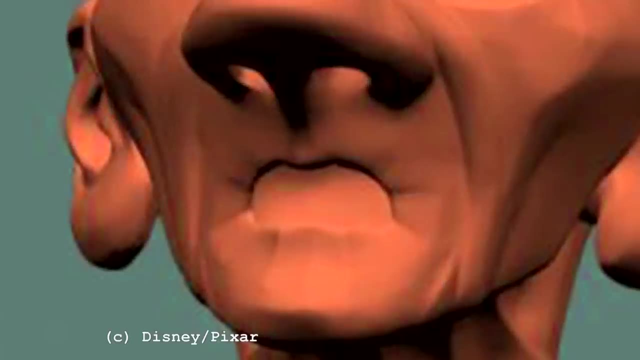 To the untrained person, which I very much am, it doesn't seem very subtle. It seems like anything you feed into this process will just kind of get blob-ized in the same way. Everything will get turned into this kind of generic blob. Is there more nuance to this than what it looks? 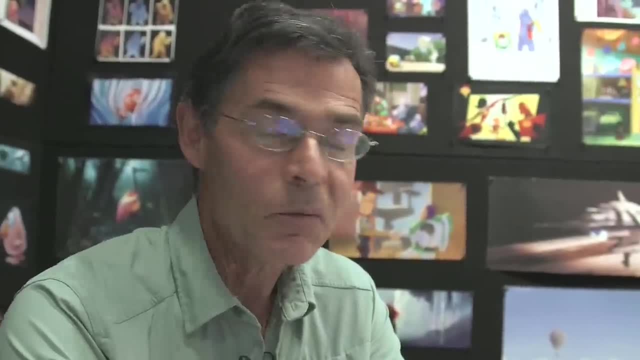 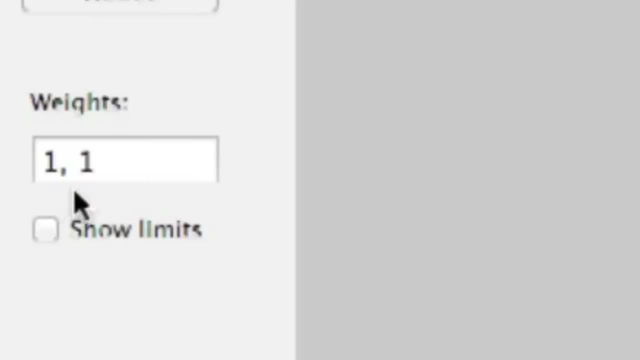 like, Or does everything turn into a big bleh? Well, there is some nuance, There's some magic numbers involved, So let's get a sense of what those numbers are. One pair of magic numbers are one one here. Those are the weights that I used in this average average. 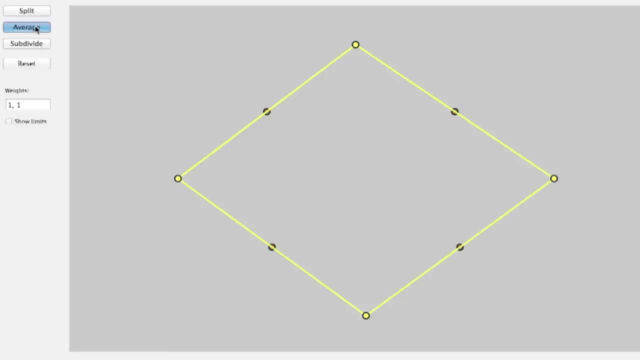 And those are magic, because you can show that a nice thing happens in the limit of this subdivision. So this one one means he's going to go to a spot that is one part of where he is now and one part of where his right neighbor is now. Okay, so let's do that, Let's, let's. 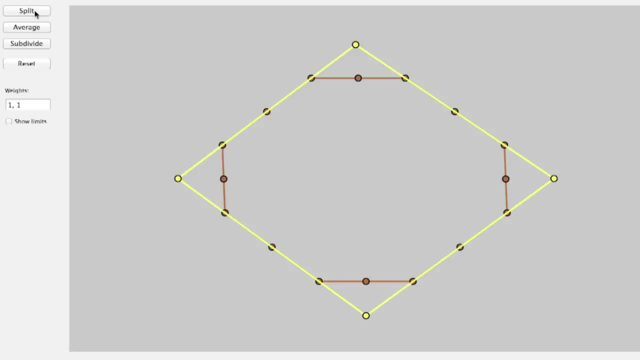 each stage is split, followed by average. So there's the split. So when he moves according to the one rule, he's going to move from where he is now to here, And this guy's going to move from where he is now to here, and so on. So we'll see that And we just keep repeating that process. 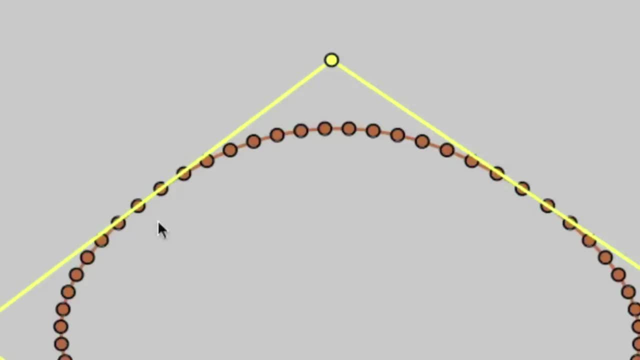 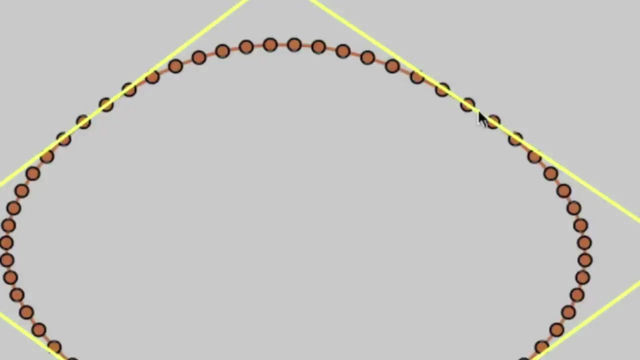 And a beautiful thing happens In the limit. you can show that this curve is. there's a parabolic arc that sits in here And there's another parabolic arc that sits in here, And those two parabolic arcs meet with a smooth derivative, a smooth tangent line. at this point. 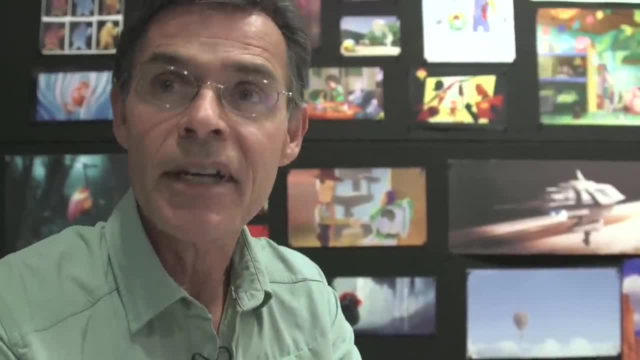 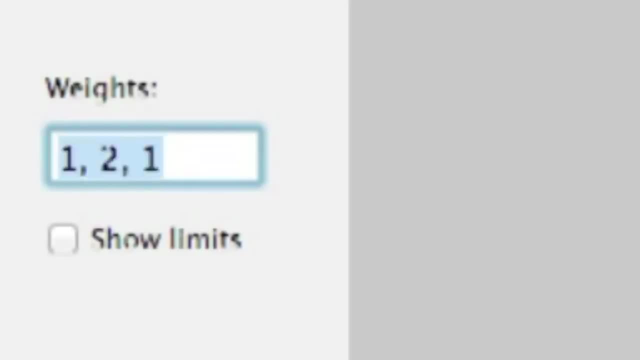 And that's all just an emergent property of this subdivision process. There are some other magic numbers I can use. For instance, if I use one, two, one, So I split as before. Now, if I use the one, two, one rule, this guy's going to move from where he is now to two parts of where he is now. 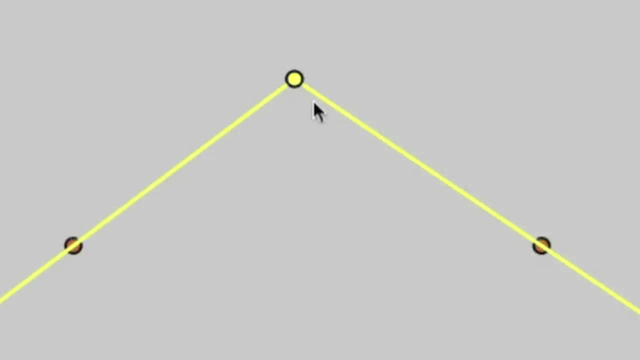 One part of his left neighbor and one part of his right neighbor, So it's one, two one. So he's carrying more of his weight. Yeah, exactly, And so if I average with that set of weights, I get a shape like this: I continue to split and average Again. something really nice happens. 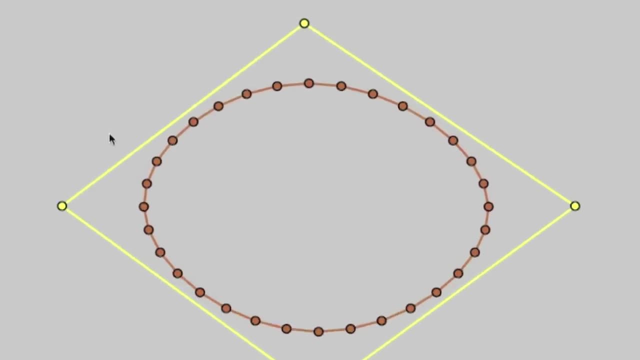 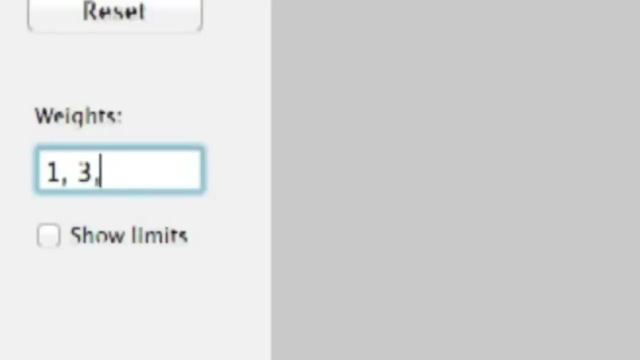 When we use the one one rule, we got piecewise parabolas which are degree two curves. Here we're going to get degree three curves in the limit And if I pick weights one, three, three, one and do this process, it turns out you get degree four curves. And this pattern is 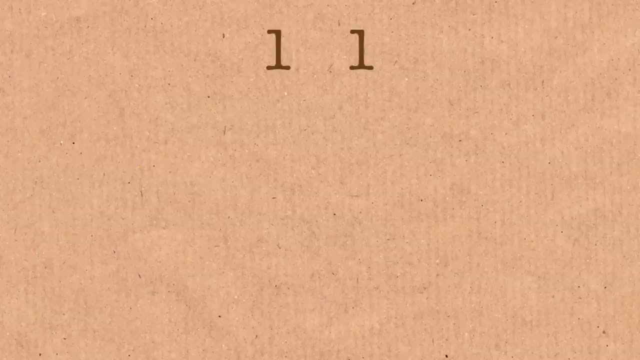 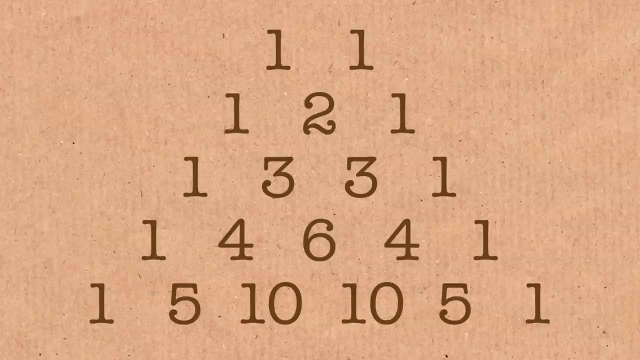 I think probably familiar to many of your viewers. One one, one, two one one, three, three one. Those are all rows of something called Pascal's triangle. So what we're learning here is that, if you pick your weights carefully, that is. 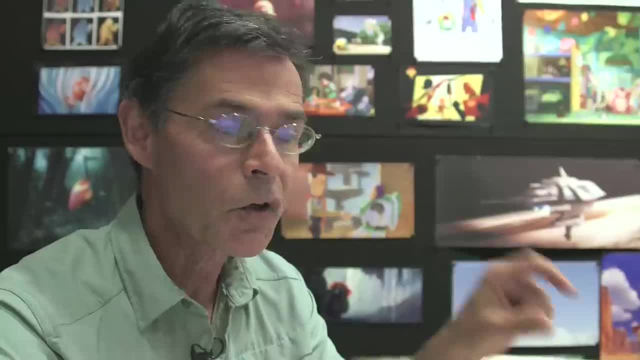 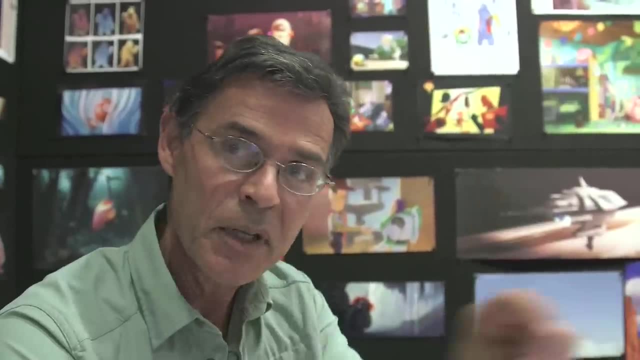 from rows of Pascal's triangle. the curves that you get in the limit are nice and smooth and they're polynomials, And the degree of the polynomial is given by how deep into Pascal's triangle you pick your weights. But you don't have to pick them carefully, You don't have to. 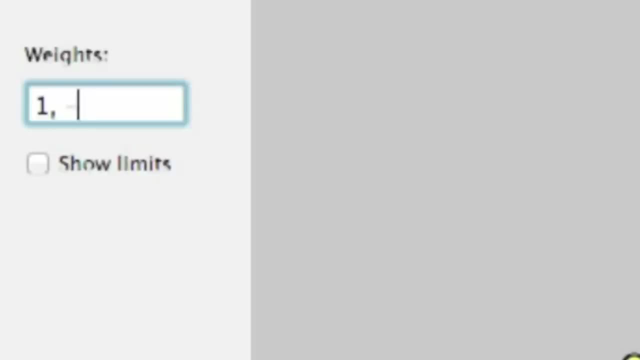 pick your weights carefully. I can. in fact I don't even have to make the weights positive. So suppose I pick rates one minus two and three. So I split as before, And now this guy's going to go to a point which is minus one times himself, one times his left neighbor. 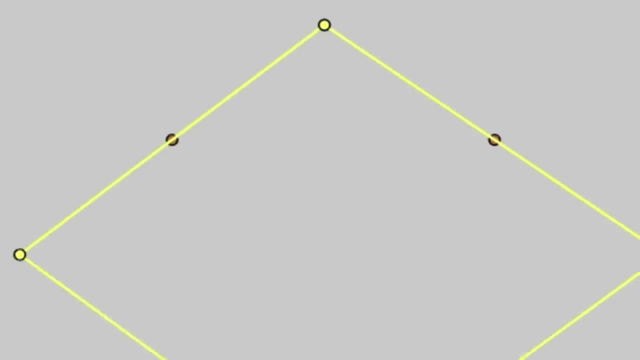 and three times his right neighbor. I've got no idea what's going to happen. Yeah, let's see what happens. Oh, OK, something interesting, Let's continue. We'll keep doing that. So what we're seeing here is in the limit. if you don't pick your weights carefully, you get. 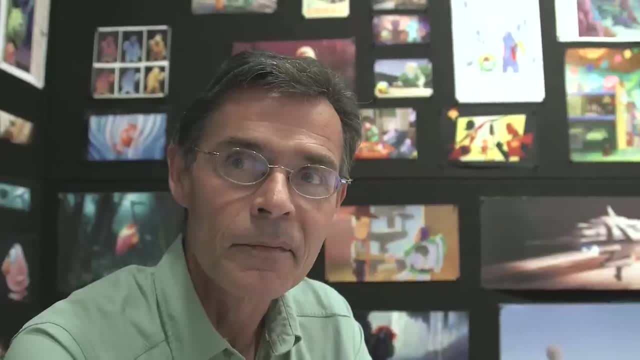 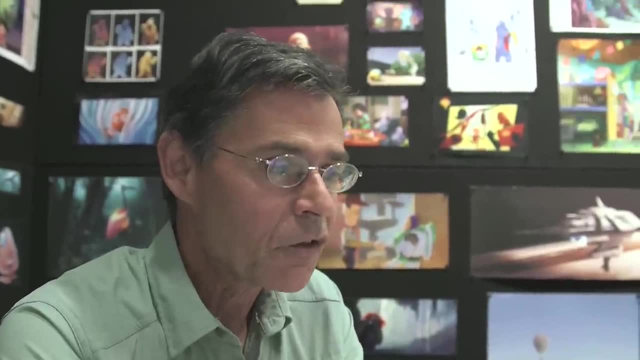 the same thing. You don't pick your weights, but you pick the ones that are not. you know you didn't pick yours, So let's try to pick the ones that are not, or you'll pick the ones that aren't and you'd pick the ones that are only somewhere. In fact, it's a fractal. 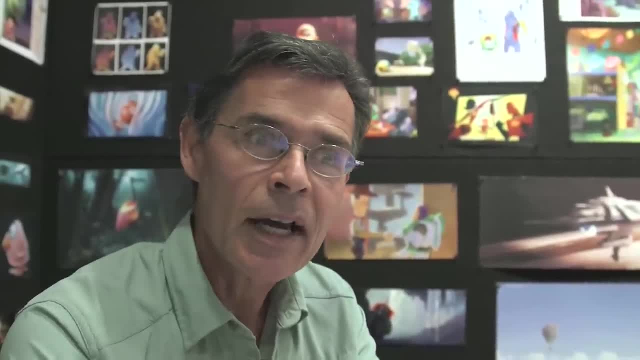 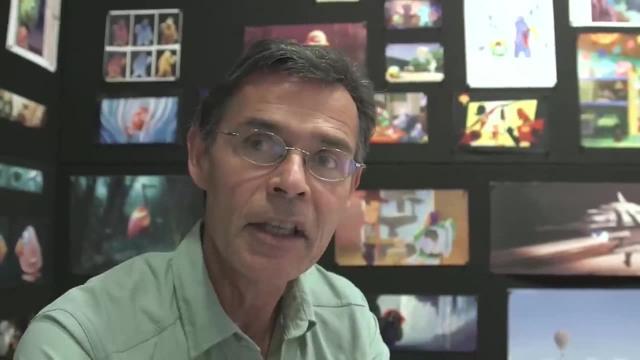 So when I watch one of your films, which one is the right one? Which one creates the surfaces that make you happy? Well, it turns out that for surfaces, this Pascal's triangle pattern doesn't work anymore. You have to use a different set of. 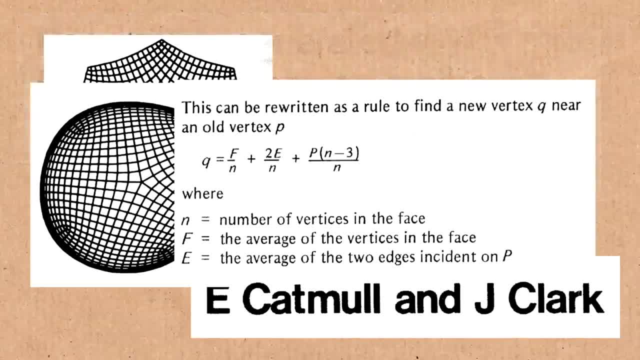 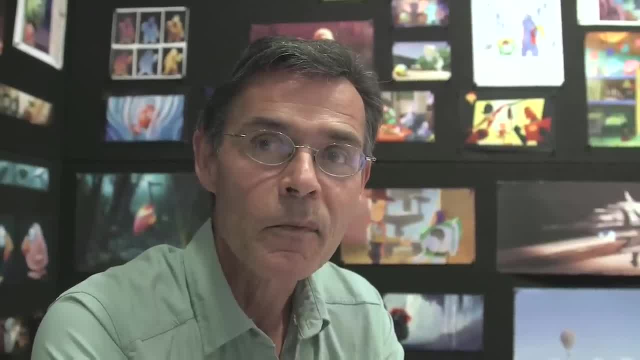 by Ed Catmull 40 years ago. Ed's the president of Pixar. Do we know? are those like? are they like fractions? Are they? what numbers are they? Are they like one, 1.7 and 3.92, or? 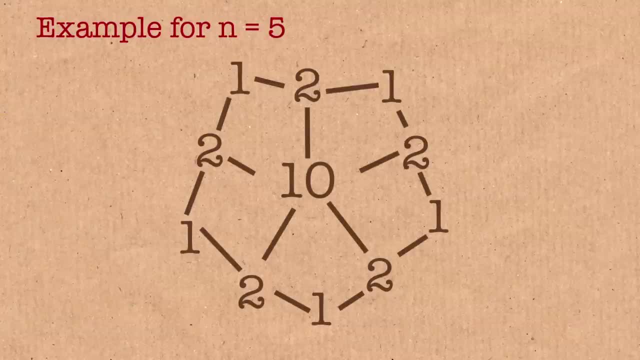 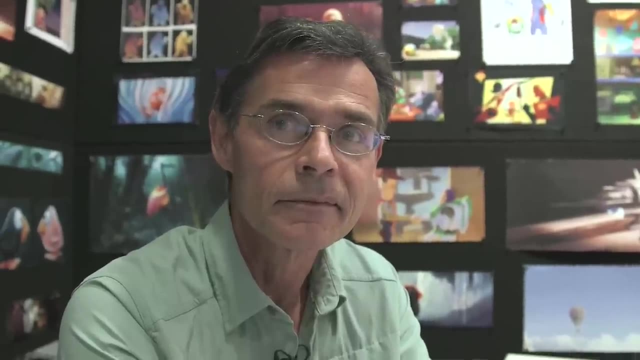 Well, I don't remember them off the top of my head, but there's a simple formula that is now well known. You can find it on our website. So when you've got your 3D object, they're the ones you plug in and then bang. 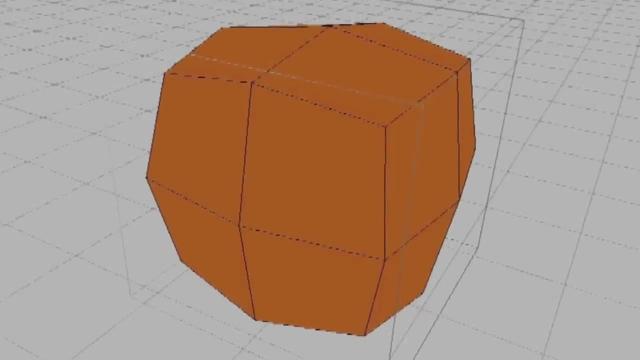 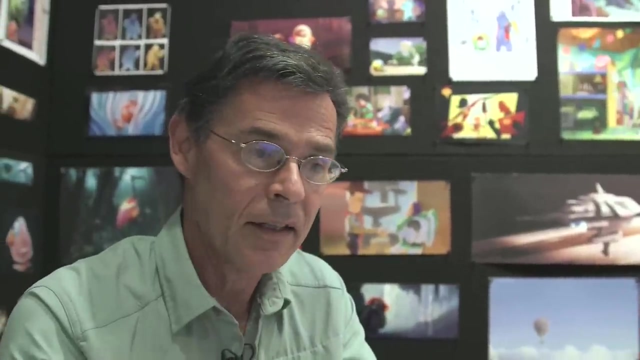 Yeah, exactly So what I was doing- the subdivision with the cube. we were using those very carefully constructed weights that Ed discovered. We do the subdivision process a few times and that gets us points that are kind of close to where they would go if we did it. 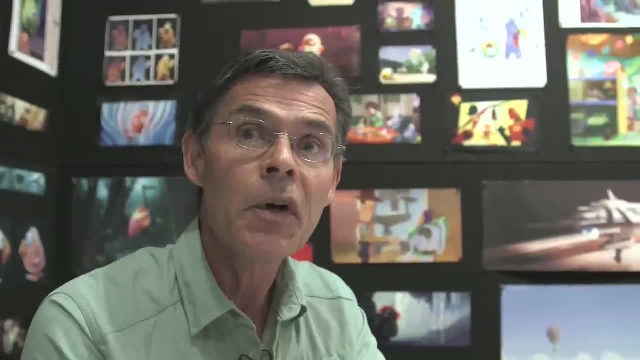 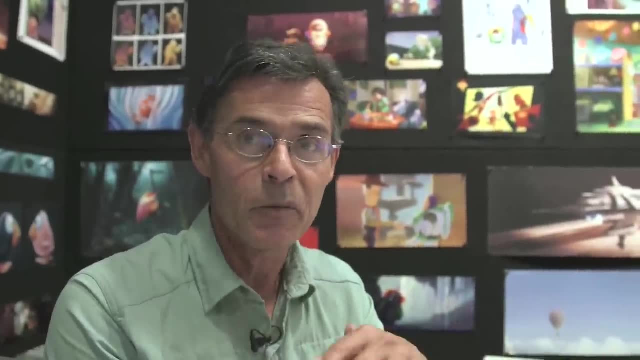 an infinite number of times. But on top of that there's a few tricks that we use to figure out exactly where they're gonna go Mathematically. we think about what would happen if we did it an infinite number of times And it turns out that we can write down exactly. 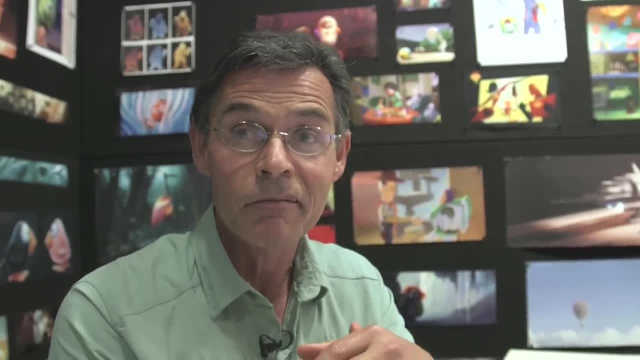 what happens if we did do it an infinite number of times. That's cracking up the paper, Yeah, so let's see how that works. All right, great, And let's start with an observation here. So I'm gonna go back to the simple one-one rule. 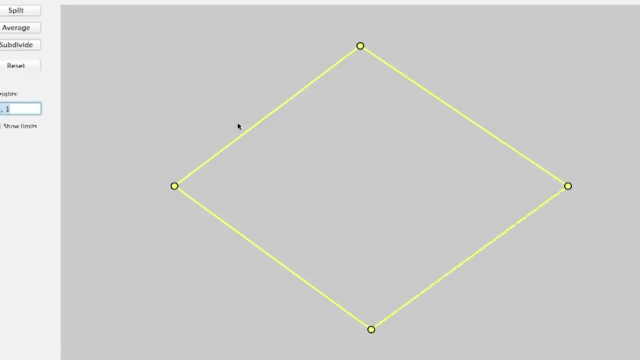 that we had earlier And watch what happens on, say, this leg of the polygon. So I'm gonna split an average And notice that what happened here is that I still have two points on this polygon leg. They're just a little bit closer. 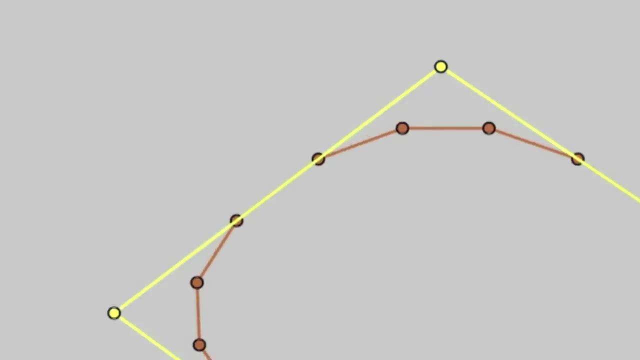 If I split an average again, again, I get two points on this leg. They're just a little closer together. If I do it again, again they're closer. So what's gonna happen if I do this an infinite number of times? 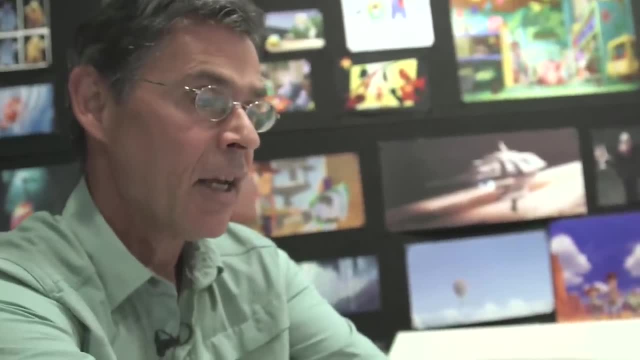 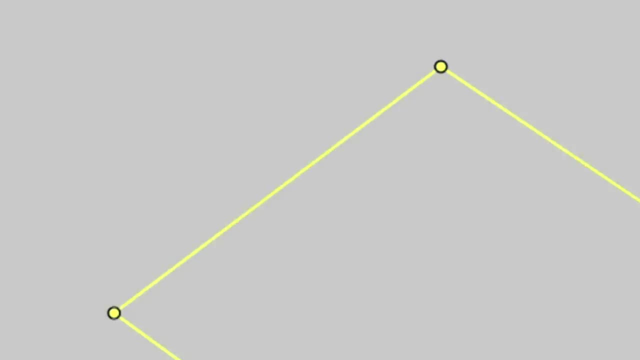 Well, these two points are gonna get closer and closer together. In the limit they'll be on top of each other And the location where they converge is the midpoint of the original leg. So without doing any computation at all, I can determine very quickly that these four blue points 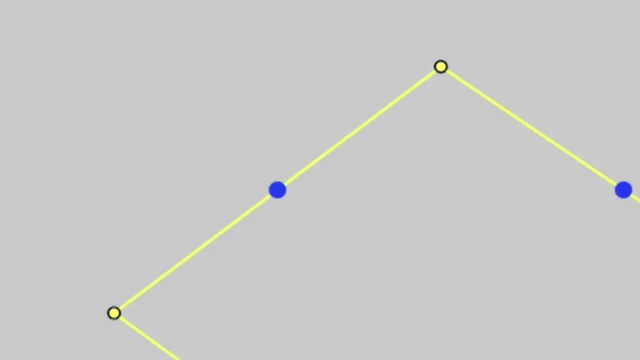 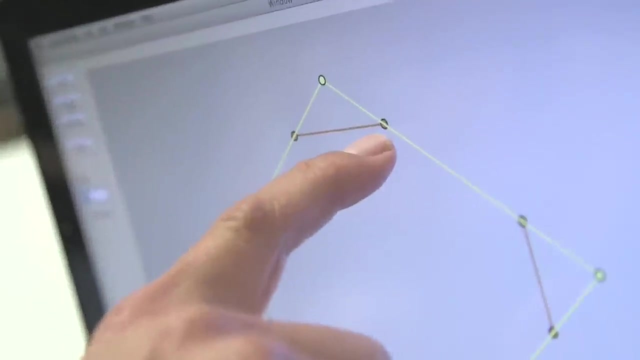 are on that limit object. And the nice thing about this is that that observation is that it holds at every stage of subdivision. Watch what happens on this leg of the polygon. So this leg wasn't in my original arrangement, but it got introduced after the first stage. 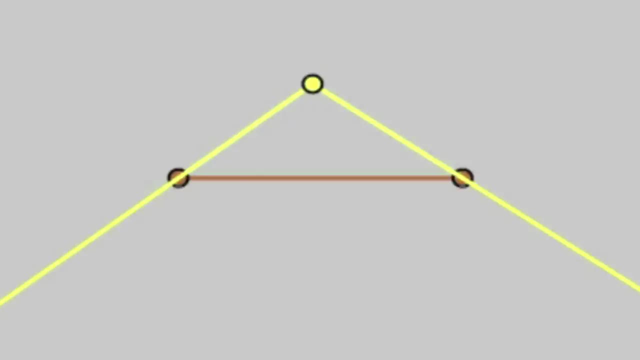 And as I split an average, we're gonna again see two points on this same line. They just get closer and closer together as I subdivide And again they're gonna converge to the midpoint of the leg when it was first introduced. 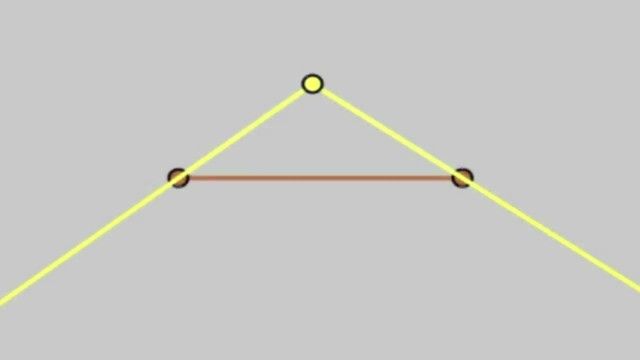 So let's go back to that arrangement here. So I know that the midpoint of this leg is also on the limit object. So after one stage of subdivision I already know eight points exactly. You refer to this thing called the limit object. That's the finished product. 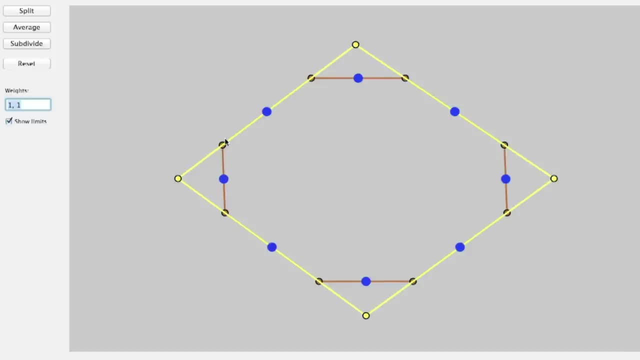 That's the finished product, right? So it's the mathematically perfect version. And now I've got eight points that are on the mathematically perfect curve. Computing what happens in the limit becomes a little bit more delicate when we look at one of these other rules. 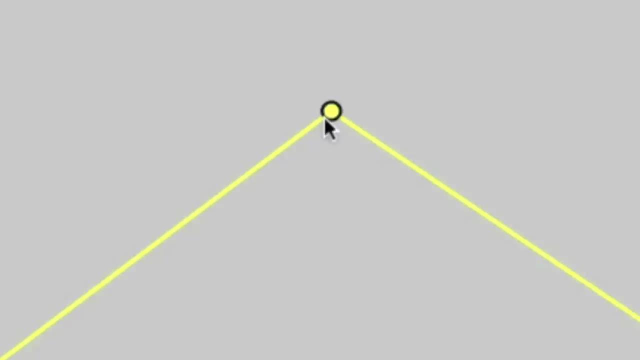 like the one two, one rule. So let's see if we can track where this point goes. as I subdivide, We're using a one two, one. now, This is a one two, one rule. So if I split an average, 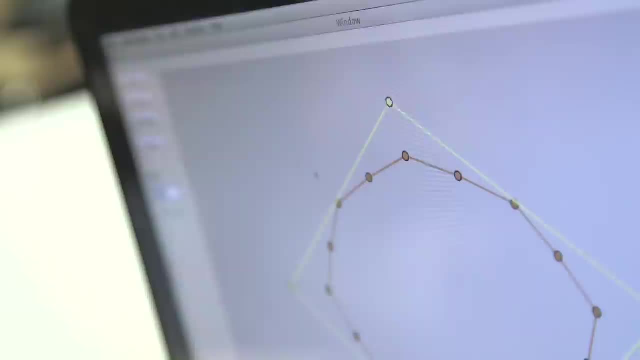 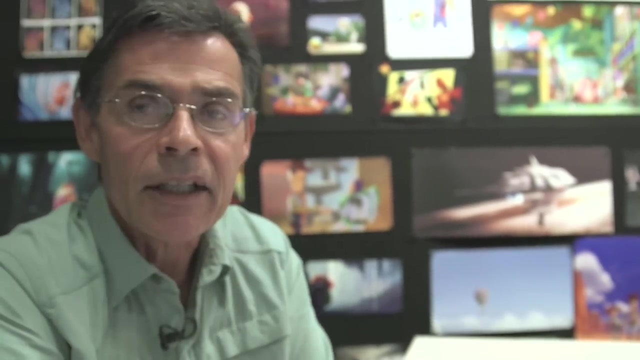 okay. so he moved some distance. Let me split an average again. He's moved a little bit more. It's not exactly clear where he's gonna stop. He's not on the limit object. He's not on the limit object yet. 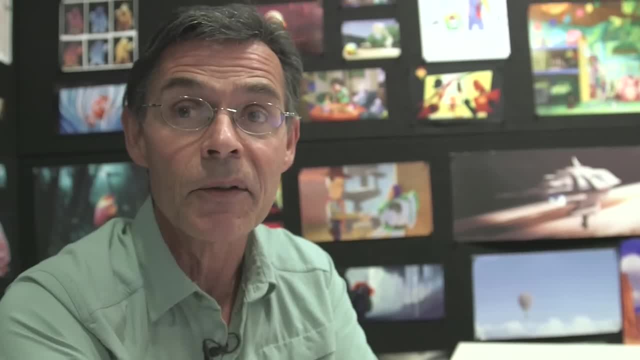 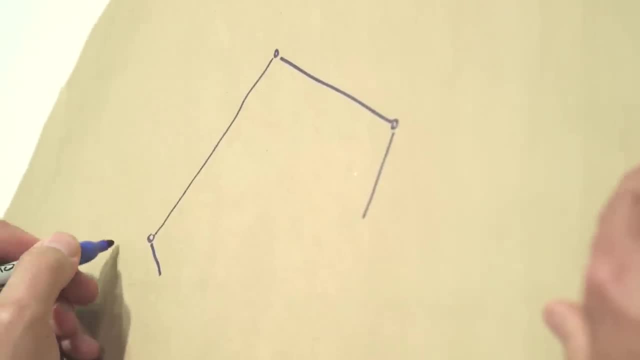 So, but yet we can compute exactly where he's gonna go with some other magic numbers. Let's take a look at how that works. I'm gonna draw a little piece of my curve- my original polygon. And since this is my original polygon, 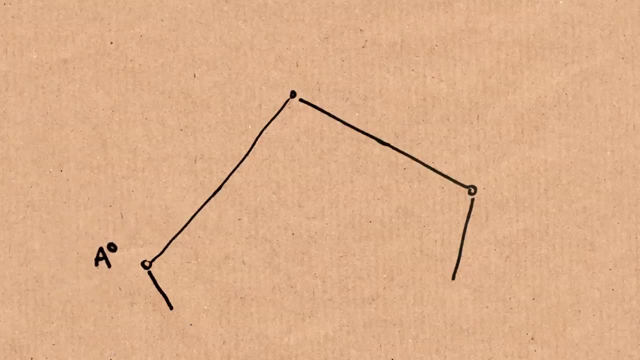 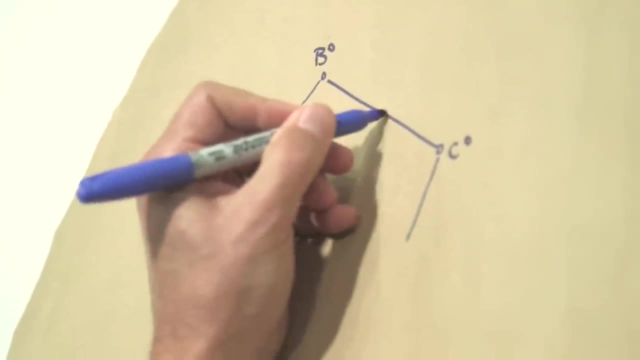 I'm gonna use superscript zero. So a is super zero, b is super zero and c is super zero. So that's before subdivision. If I subdivide once, I get some points that are gonna sit in here And I'm gonna call this guy a super one. 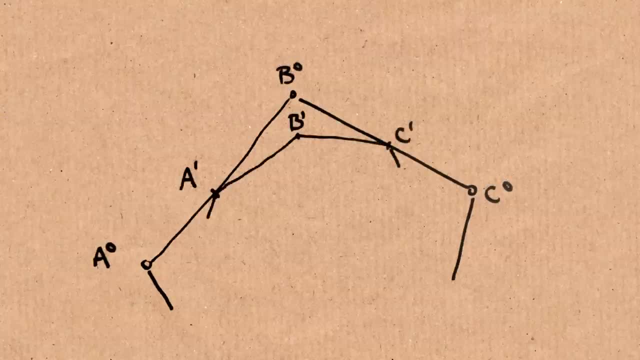 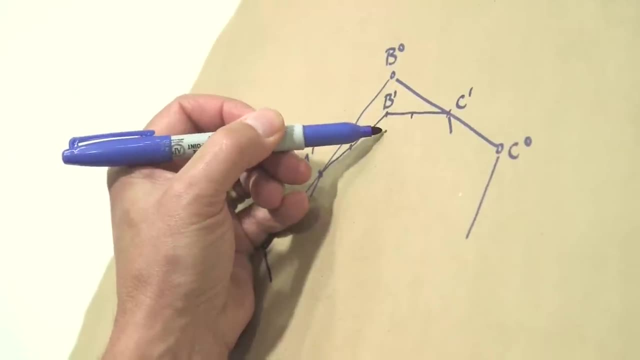 b super one and c super one, And if I subdivide it again, I get some more points in here And what we wanna know is: okay, here's b zero, here's b one, b two's gonna be someplace. 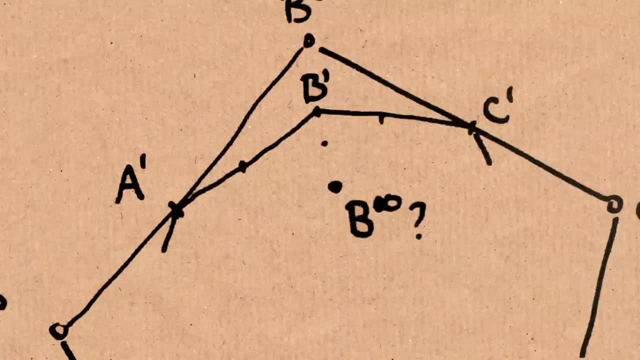 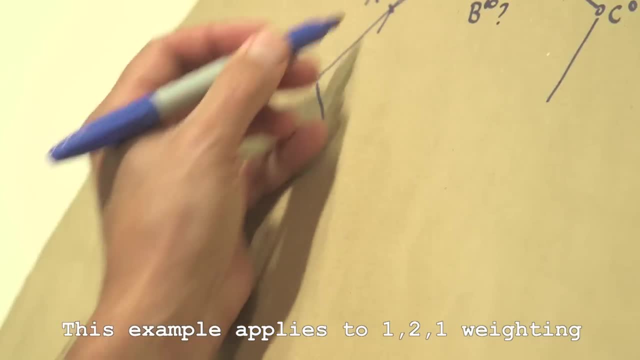 The question is: where is b infinity? We'd like to figure out where that is Turns out. we can answer that question And to do that, I'm gonna write down a few things I know. Well, one thing I know is that a super one is just on this midpoint. 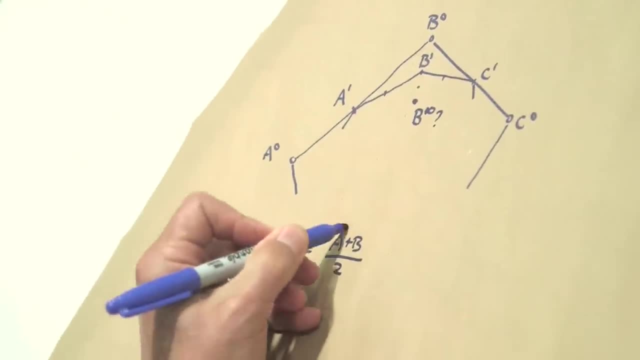 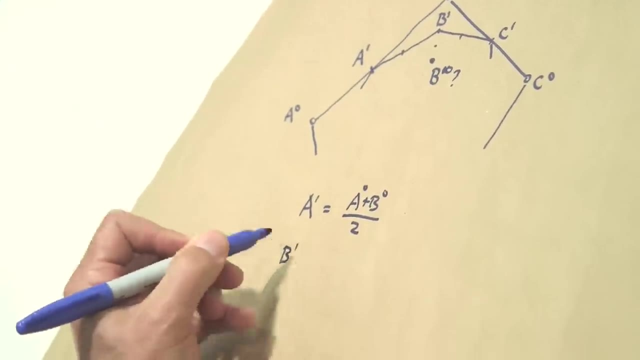 So I could write that as a plus b over two and these are super zero guys, my original things. If you work out the algebra of the splitting and averaging using the one, two, one rule, you can see that b super one is a super. 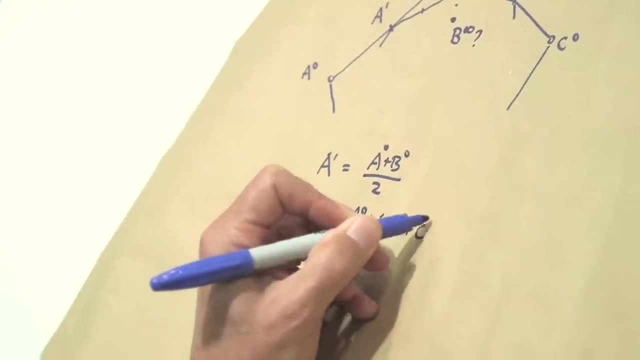 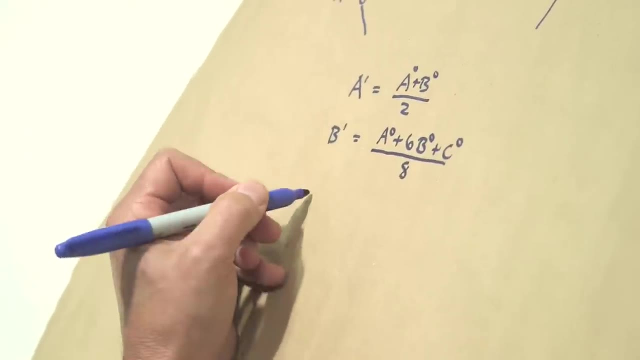 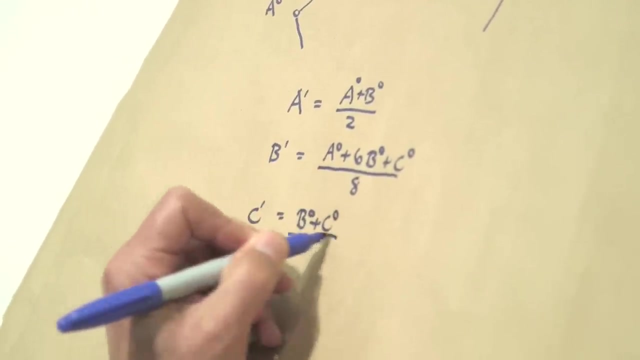 zero plus six, b super zero plus c super zero Divided by eight. so that's just unwinding the split and average process, And then c super one again is just the midpoint on this leg. So that's b super zero plus c super zero over two. 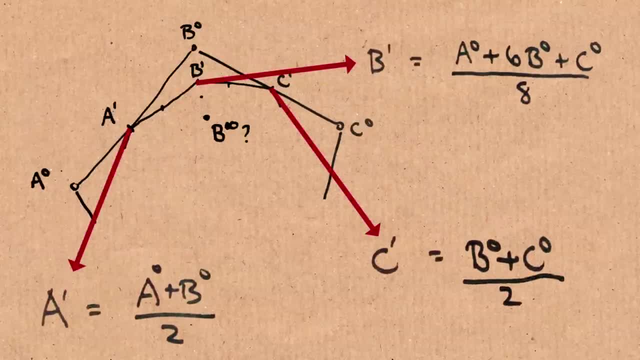 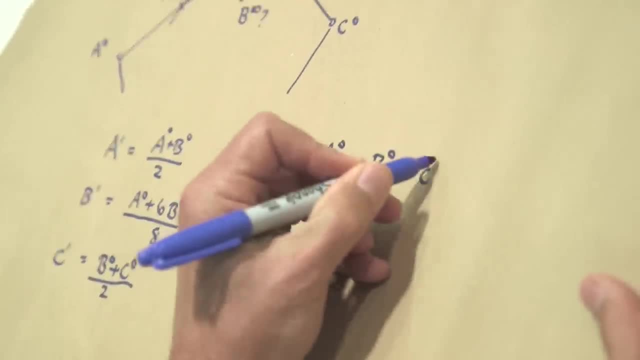 Okay, well, that isn't obviously helping us answer the question of where b infinity is To do that. I'm gonna do something a little bit sneaky: Take a super zero and b super zero and c super zero And combine them with weights one, four, five, six and ten. 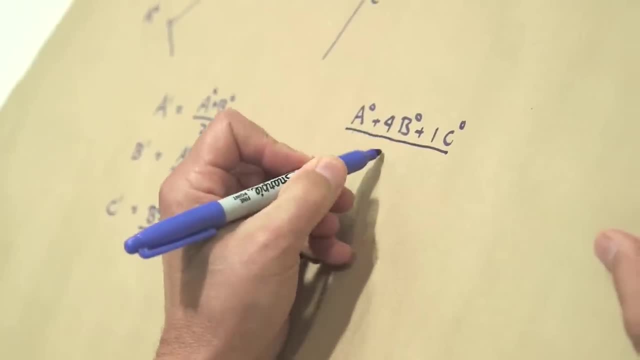 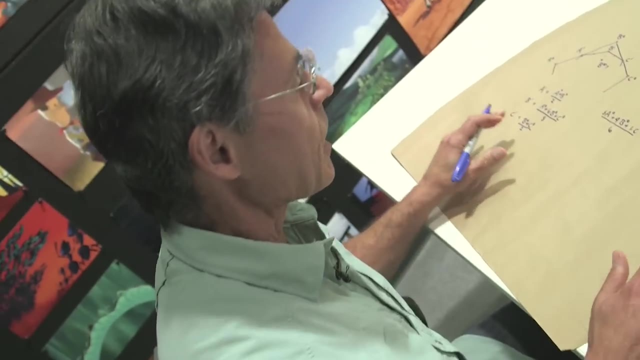 One, four and one, And we'll have to divide by six. so I'll put a one there, Cuz I have kind of six things in the numerator. Where did the one, four, one come from My back pocket? 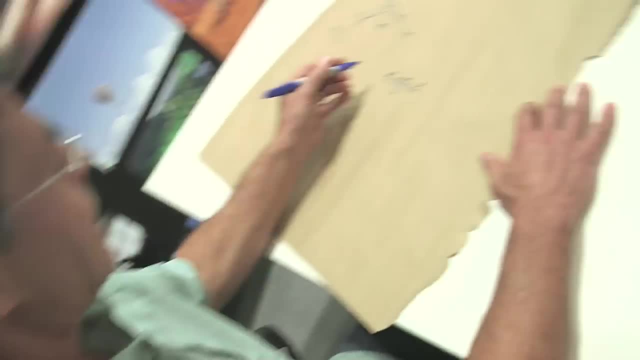 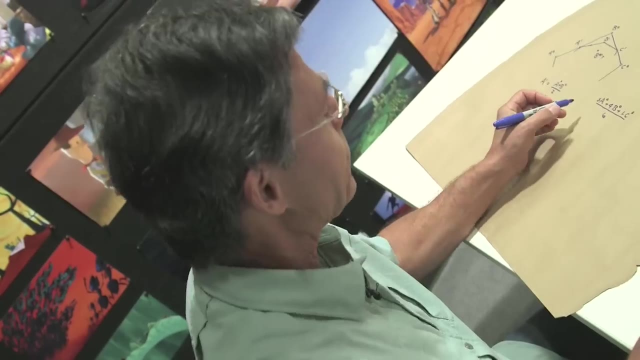 And you'll see why I picked one four one in just a second. The real answer is it came from a tool called eigenanalysis, But we don't need eigenanalysis to see what's gonna happen here. I'm gonna take that same combination and. 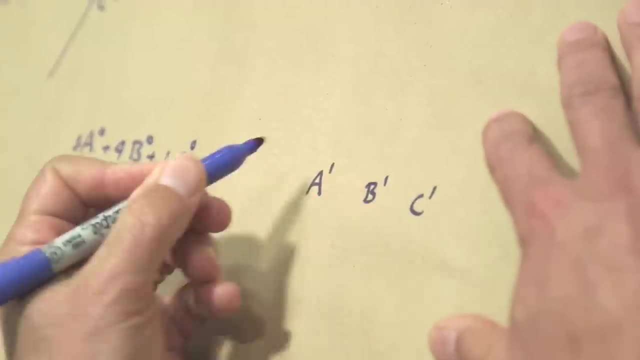 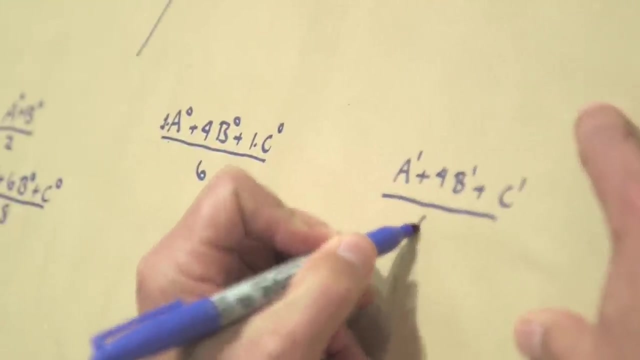 apply it to a super zero, A super one, b super one and c super one. So I get four b super one, one copy of a super one, one copy of c super one and divide by six. So now I have two expressions. 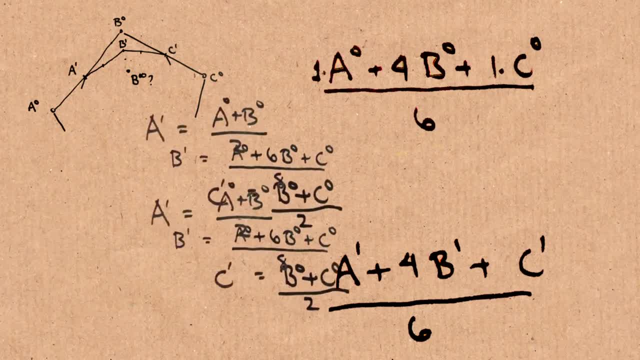 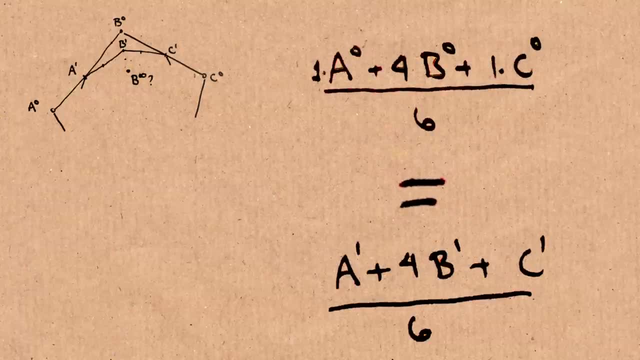 And if you take these equations over here and just substitute them in here and simplify, what you'll see is this expression is actually equal to this expression And it's only true for these weights- one, four, one- And the cool thing is that I can use that. 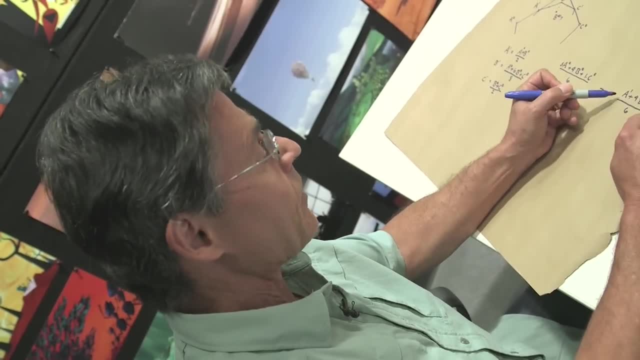 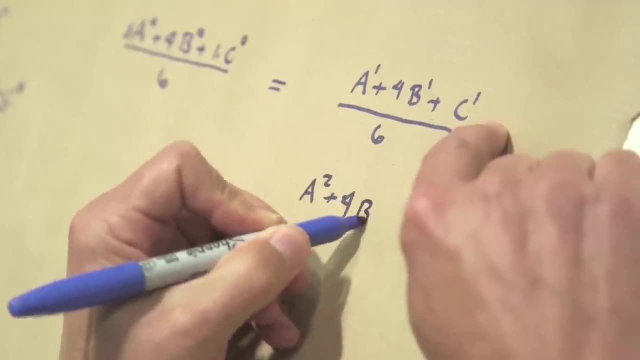 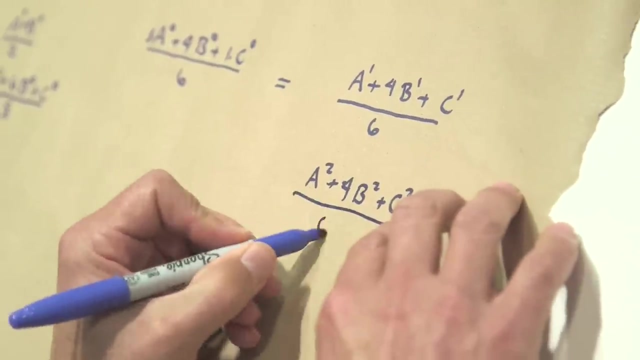 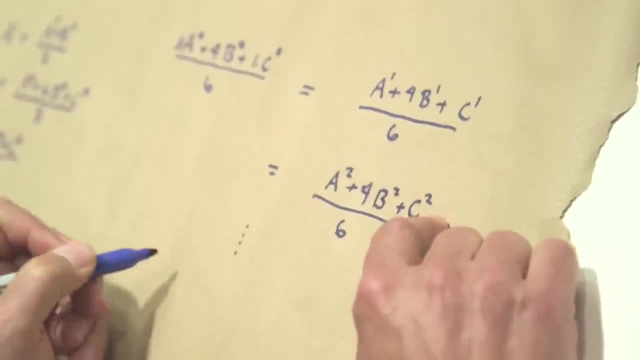 same reasoning. to figure out that, going from the super one condition to the twice subdivided condition, again applying one, four, one to the twice subdivided points over six, I'll find that these two expressions are also equal. So I can repeat this process any number of times I like. 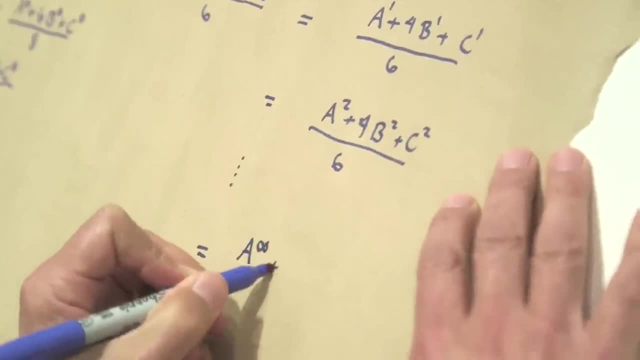 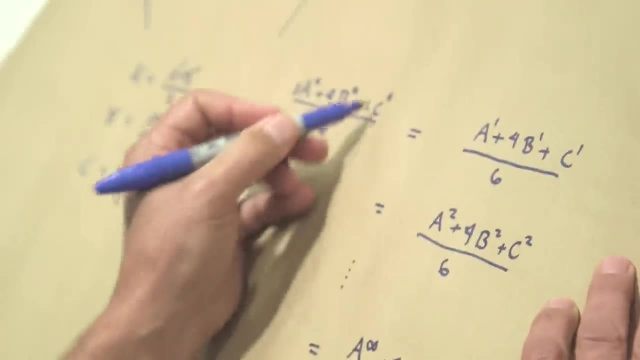 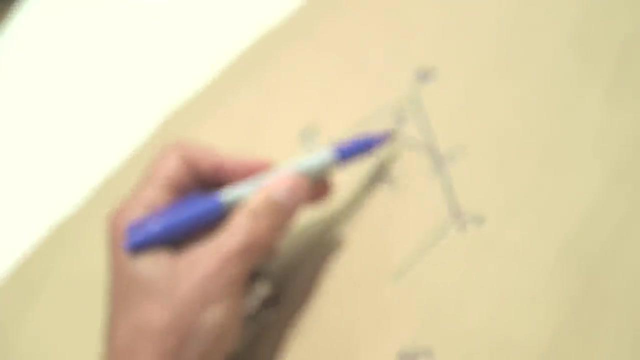 Say all the way to infinity. So I can compute A infinity Four, B infinity plus C infinity over six, And that's still gonna be equal to the expression that I had to start with. And now the beautiful thing happens. If you think about what happens to this little arrangement of three points, as you 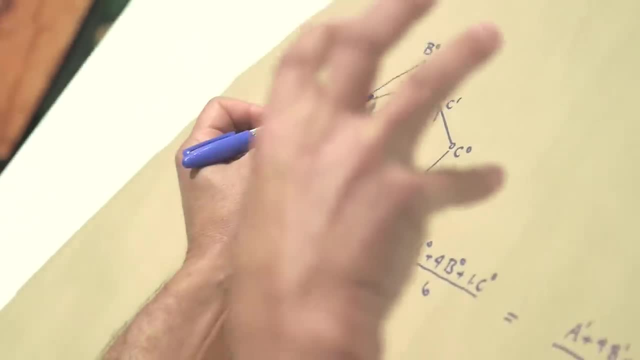 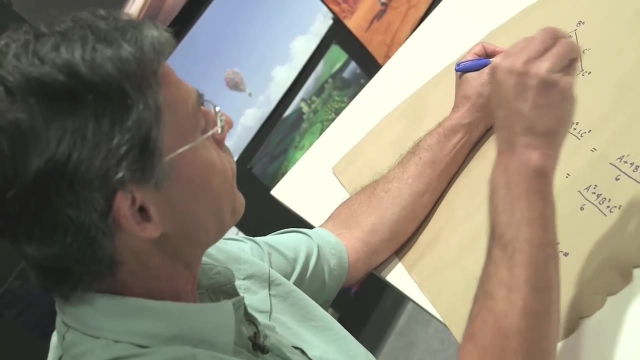 continue to subdivide those three points on. the second stage get closer together, the third stage even closer, As I do it an infinite number of times. all three of those points converge to this place: B infinity. So these are all B infinities actually.